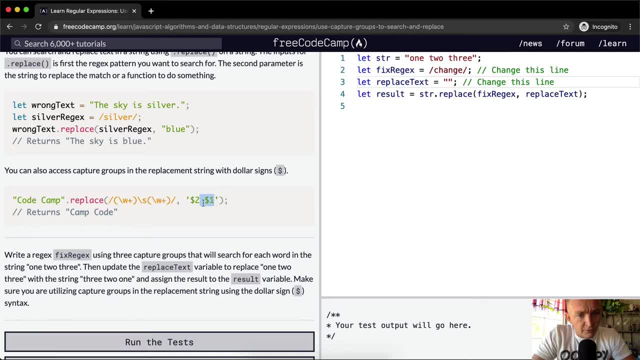 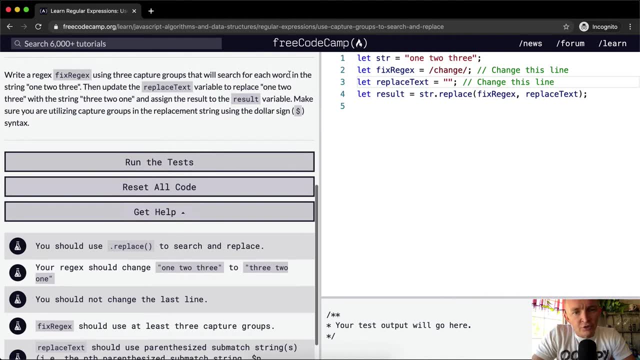 where the second capture group is in the second capture group where the first capture group is. So write a reject- fixed rejects- using three capture groups that will search for each word in the string 123.. Okay, so if we're going to search for each word, we're going to have three capture groups. 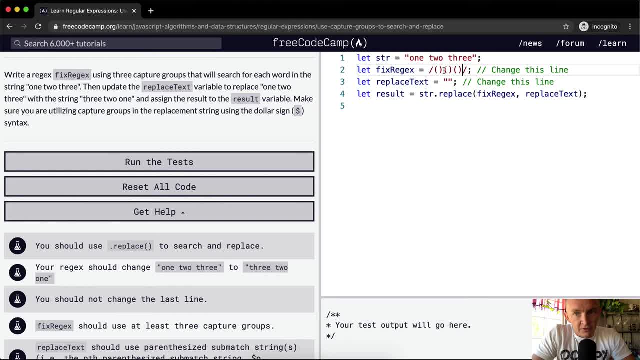 Using three capture groups that will search for each word in the string, And so the way we'll be able to tell that they're separated is with a space. So they're separated by space and separated by space, And then how do we know that their words, we're going to say they're there. 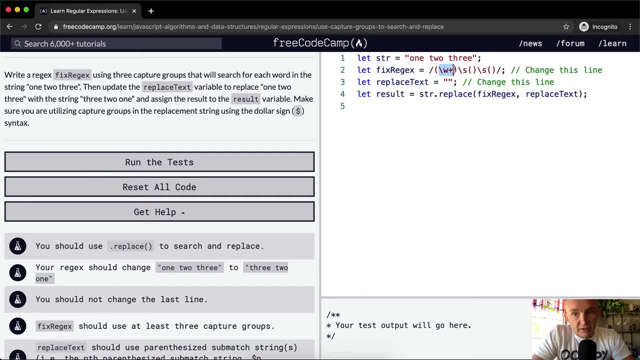 Not digits, but word and plus. So that means that we can get them of any length, right. So one letter and then as many other letters follows. for this one's two. for this one, it's the first word or letter, and then it's however many letters that follow. so this one, it's four. 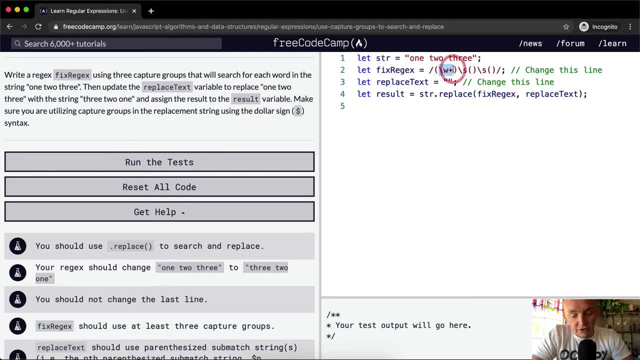 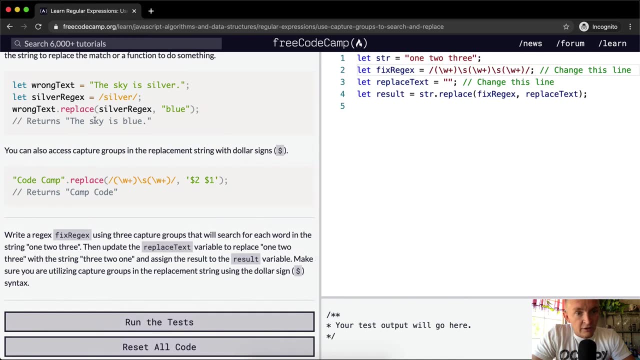 of letters that follow. we want to do this with each one of these, so i'm going to paste w plus into here. um, cool, and then, yeah, i think if we were to say, okay, so we can't really do that yet, um, two, three and then update the replace text. 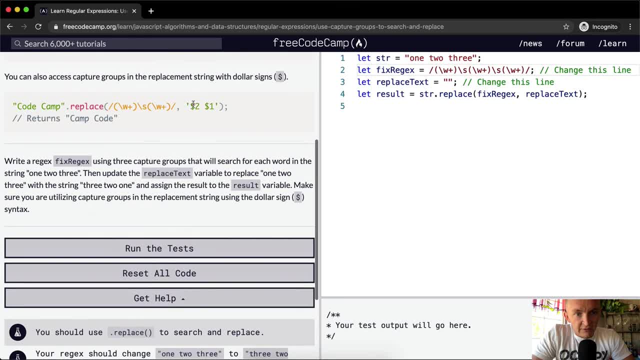 so we want the replace text to follow this convention. so we're going to come in here and we're going to say: three, oh, money sign three separated by space. money sign two separated by space, money sign one. and if we were to consolelog the result: uh, three, two, one. 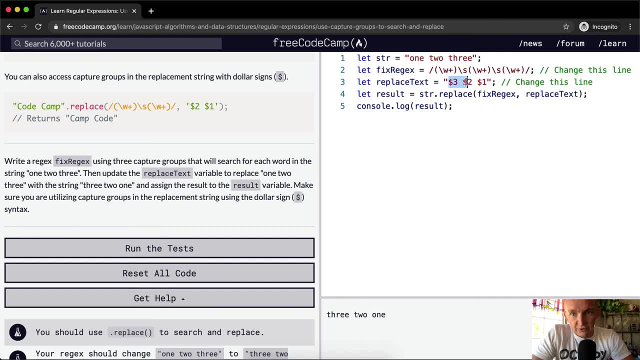 and it starts: one, two, three. so what we're doing is we're just taking the first group and putting it at the second, and then that so forth. let's play around with this. what happens if we go two, two, two, yeah then. so what we're doing is we're saying: take, replace each, each one, with the second capture. 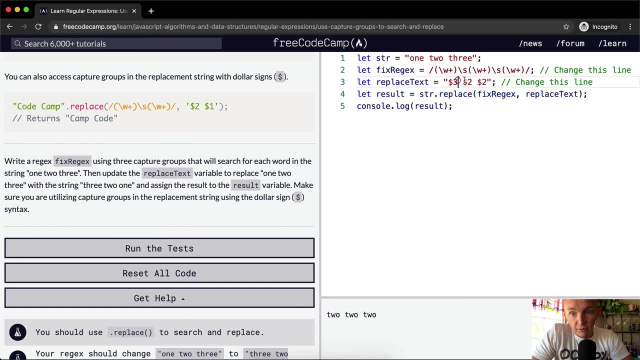 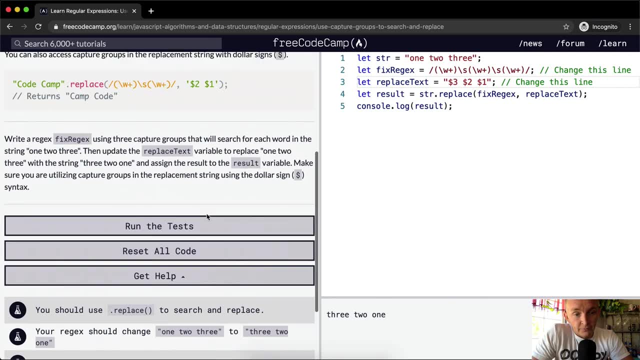 group. so with the two um, and so, yeah, so we go three two one and that gives us makes it three two one rather than one two three um. yeah, anyways, hope this passes awesome. hope you guys enjoyed this one. we'll see you in the next lesson. you.